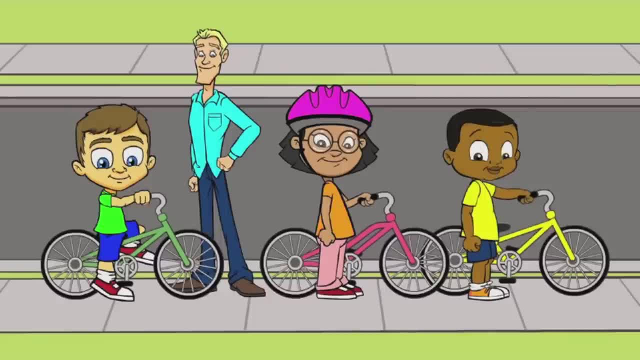 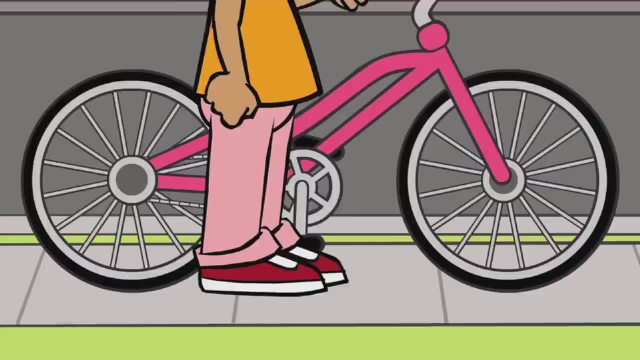 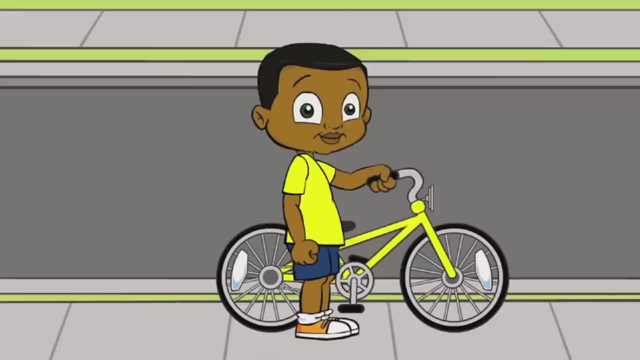 No, but you want something bright. It makes it easier for the drivers to see you, And being seen is a big part of being safe. It's also why reflectors like these are important And they look cool. But probably the most important thing you should wear is a helmet. Why? Because it protects your head if you crash. But I won't crash, I'm a good rider. Even a good rider might crash. What if a dog ran out in front of you all of a sudden? Oh yeah, I don't know. 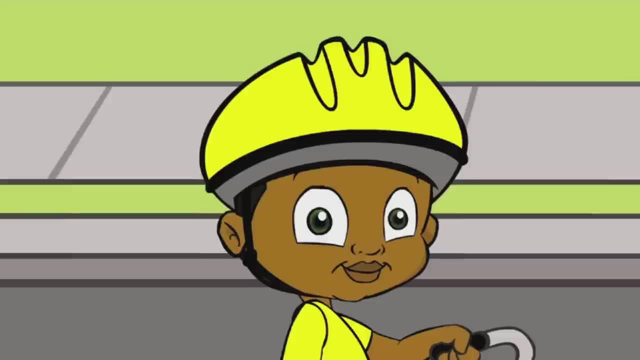 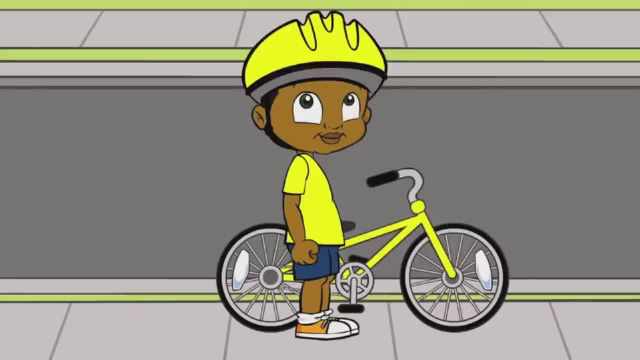 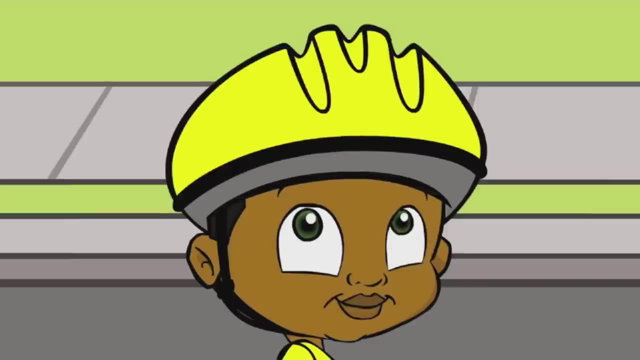 I didn't think about that. Wear it this way, Not this way, Or this way, Or this way, This way. It should fit snug on your head and sit low on your forehead like this, so you can see the edge of the helmet when you look up, And it should always be buckled. 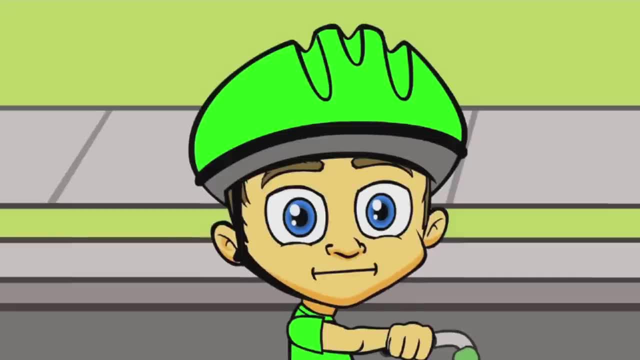 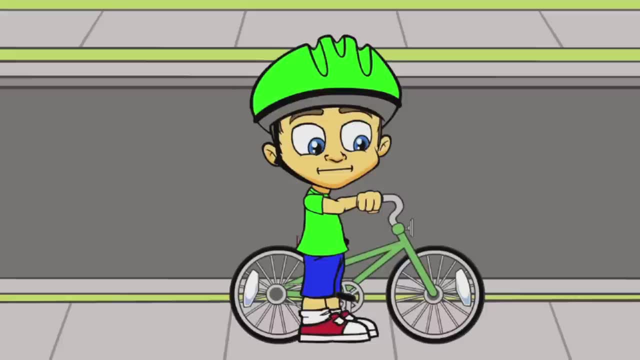 Okay, Can I get on the bike now If you remember to do one more thing. What If there's something wrong with your bike, like maybe the tires don't have enough air or the brakes don't work very well? be sure to tell an adult. 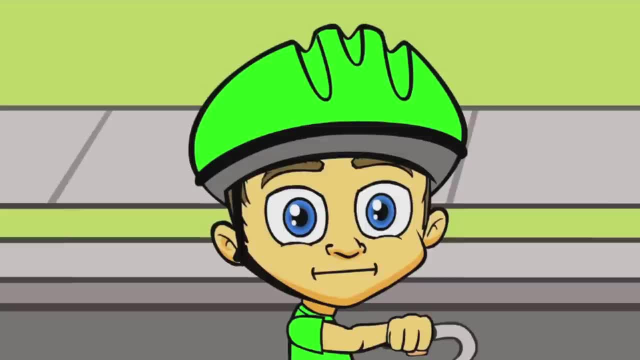 And tell them before you ride it. okay, Okay, Good. Now let's talk about the rules for safe riding. Oh man, Are there a lot? No, just a few, But they're important. The first one is ride with an adult. 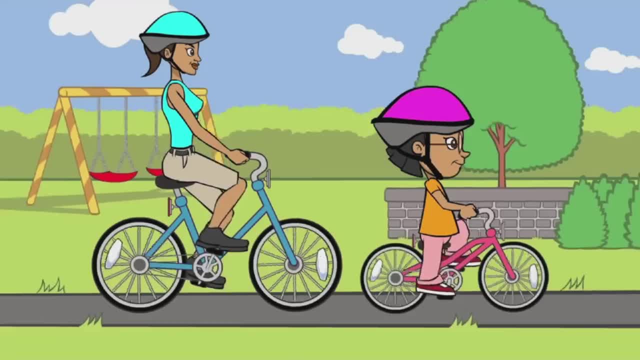 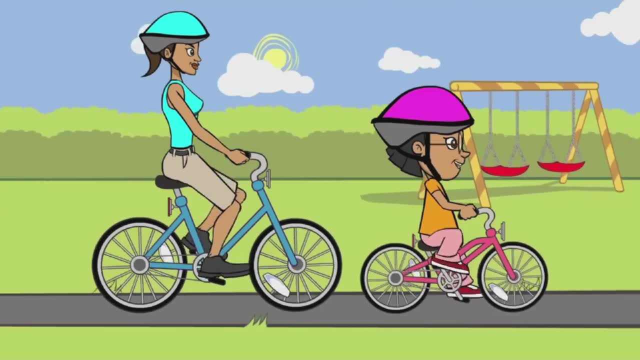 Like your parent, for example, Or with an older brother or sister. I do that with my sister. She's in high school. She helps me decide where we should ride And where's that We like to ride in the park, where there aren't many cars. 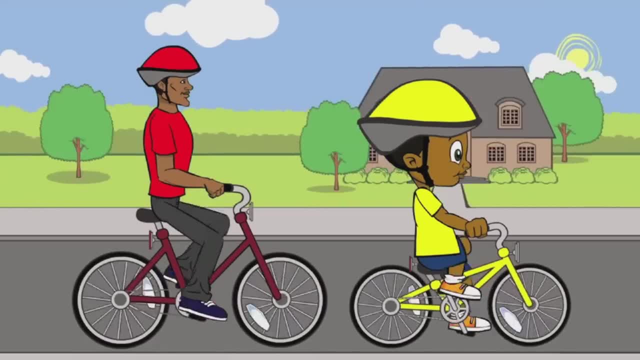 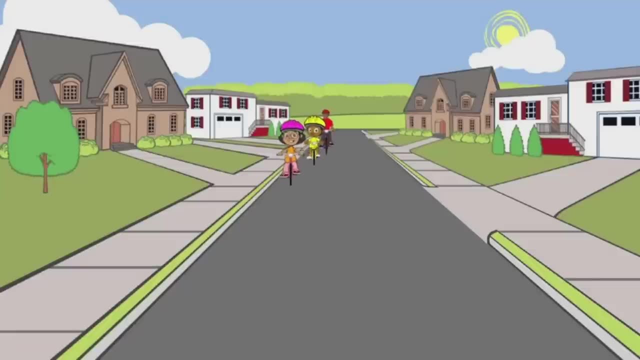 We ride on roads where there's not much traffic. Good, Those are both good ideas. And do you ride on the right side of the road or the left On the right, In the same direction the cars are going? Yes, And here's an easy way to remember that. 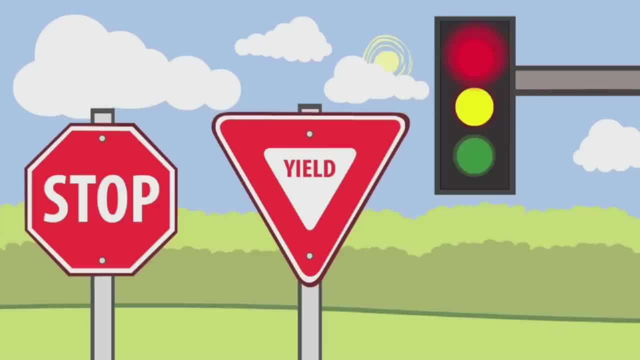 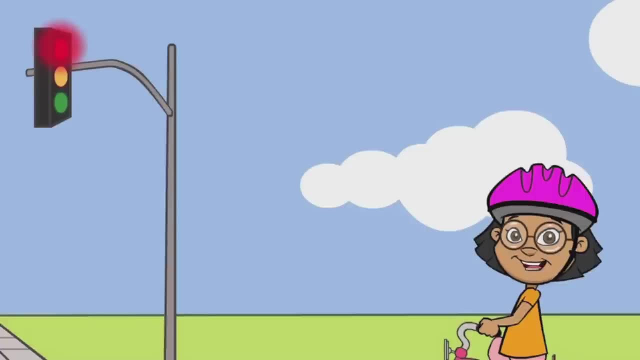 Ride right, Ride right, Okay. What else? Road signs and traffic signals: You have to do what they say. So if you see a stop sign or a red signal, You have to stop. Yes, And, And a green signal. 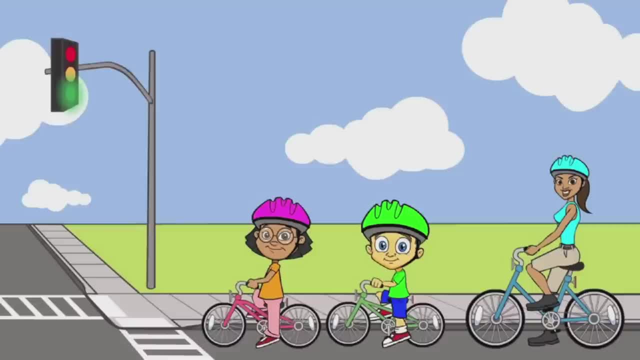 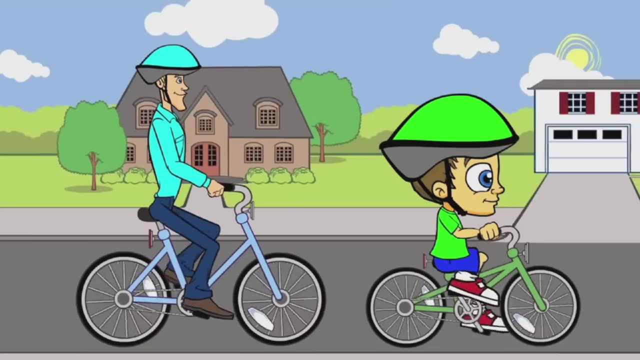 Means. you can go- It does- But you still need to use your eyes and your ears, Look and listen to what's around you. Just because you see other people doesn't mean they see you, Even if you have on a bright shirt.